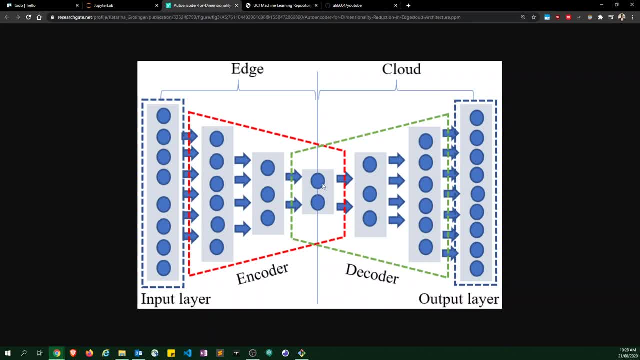 And in the encoder part you step it down towards a bottleneck point And in the decoder part we step it up towards the original size, which is also the size of the output layer Over. here we have two components in the image, and this is also what I'm going to be doing in this example. 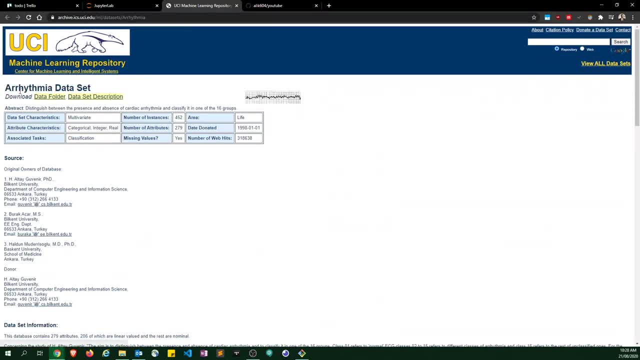 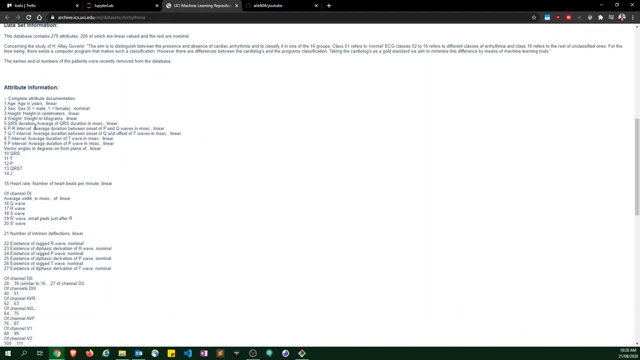 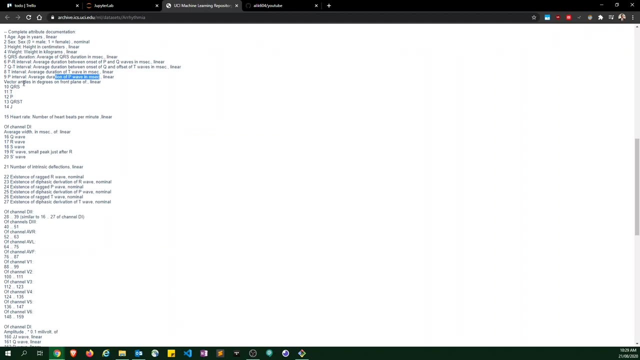 Our dataset is this: the Avifmea dataset from UCL's repository. One thing I'd like to note about it is that some variables or features are binary, others are linear, Some of them are angles in degrees and some of them are straight-up sequential. 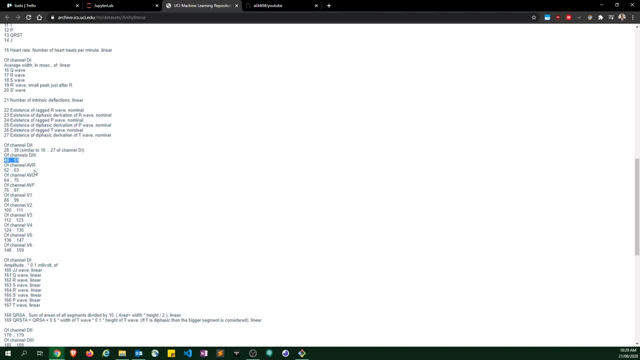 And I'm just using basically a feed-forward-net type of autoencoder. So we could, in theory, get much higher performance if we were to use something like an LSTM or something like that. But I just intentionally am keeping it simple, I'm keeping it basic and I've accomplished my goal of outperforming PCA. 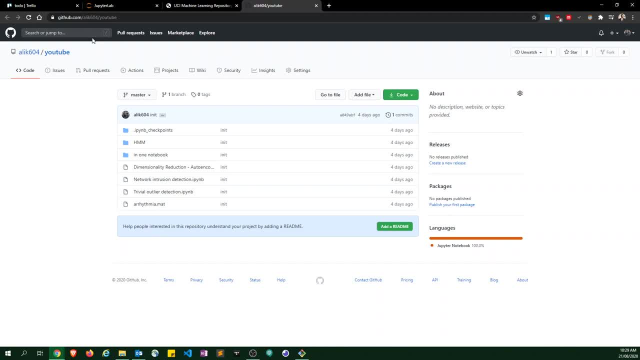 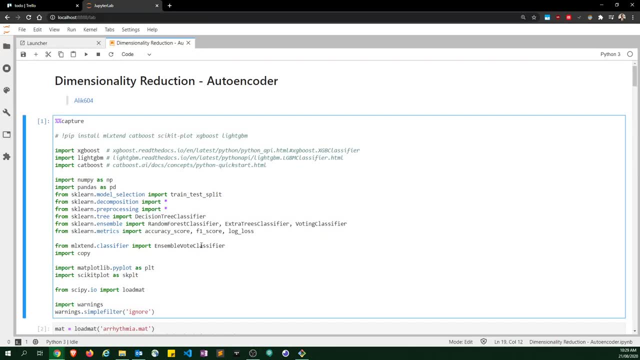 All of my code can be found at githubcom. slash a-l-i-k-6-0-4. slash youtube. Alright, so here are my input statements. I use xgboost, lightgbm and catboost. These are all gradient boosting methods. 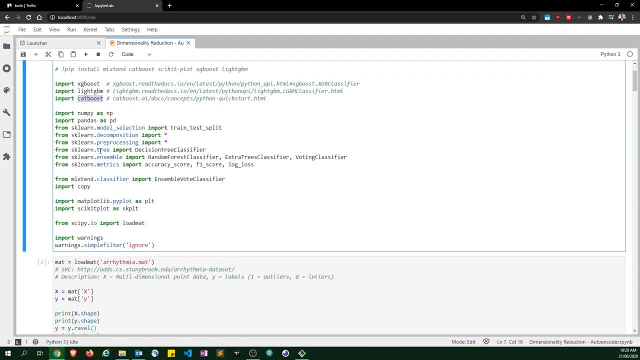 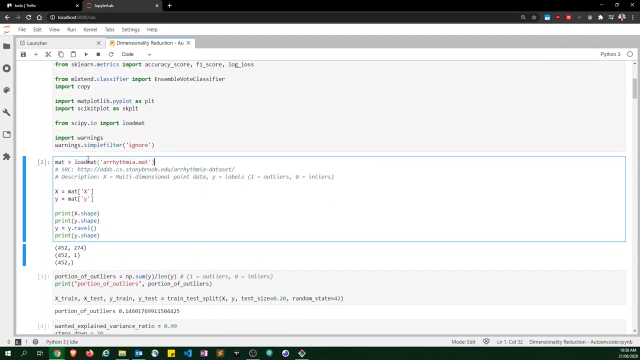 And I input some pretty normal SQL stuff. This is all for the baselining. I basically got a few classifiers to run as a baseline, so I know how my relative performance is going to be once I have my PCA versus the autoencoder. So I start off by loading up the data using loadmap from scipyio. 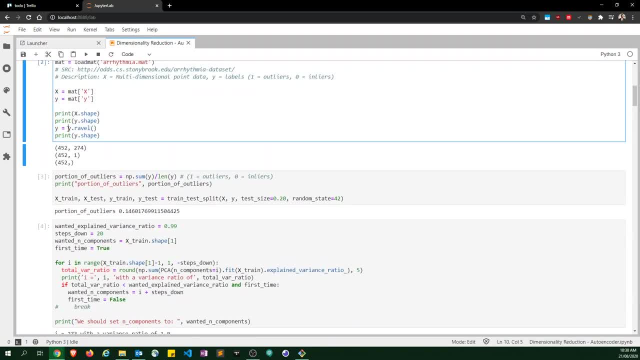 And I just unraveled the why- because it was nested. I computed the relative points of outliers. Basically, an outlier is 1.. So if I sum up all of the elements- so 0s wouldn't contribute to this, obviously- And I divide by the total number of data points, I would find out the percentage that I have of outliers, also known as the contamination. 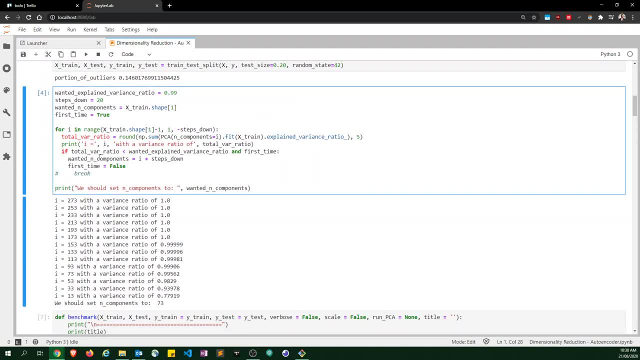 I run a quick for loop just to show the explained variance ratio of PCA across the different number of components. Basically, I take the PCA with i components, I fill it to my data, I get its explained variance ratio. I sum up all those ratios. 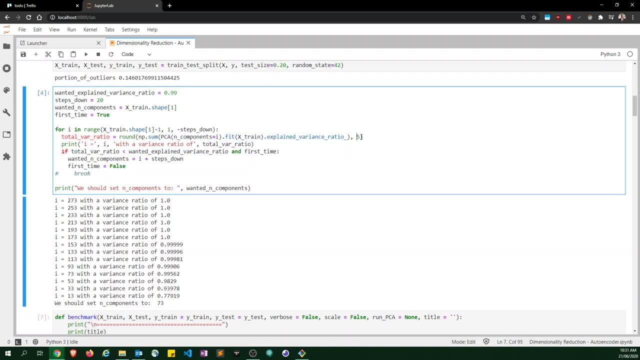 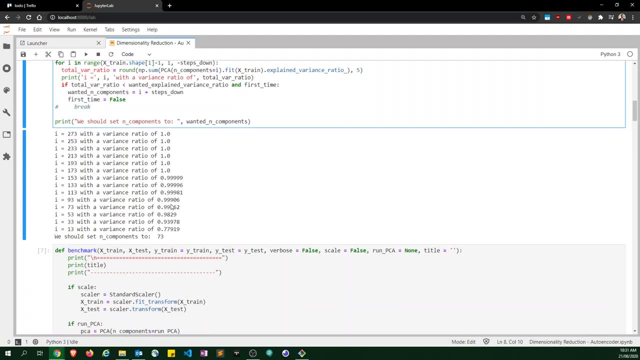 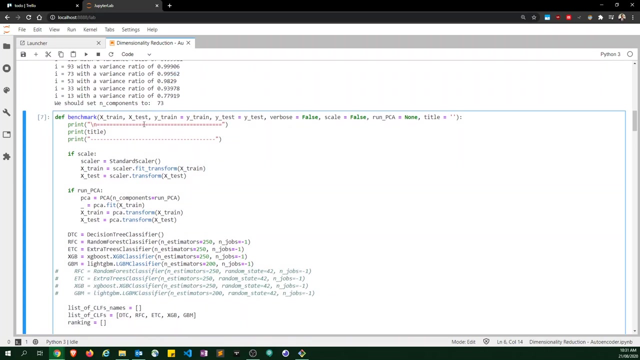 And I print it with the number loaded to 5 decimal points And I found that 75 components would give me an explained variance ratio of 0.99.. I wrote this quick benchmark function. It takes in the x-train, x-test, y-train, y-test. 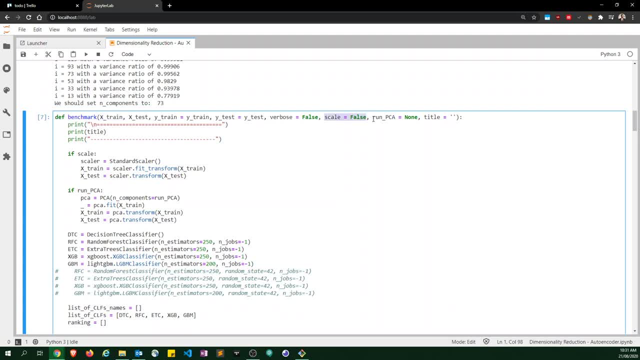 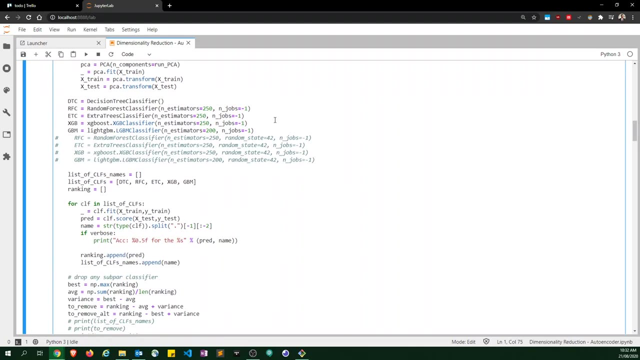 A parameter for whether we want our data scaled, A parameter which is an integer for whether we want, for whether we want and if so, how many n components to have on our PCA, And we give it a title And we give it verbose. 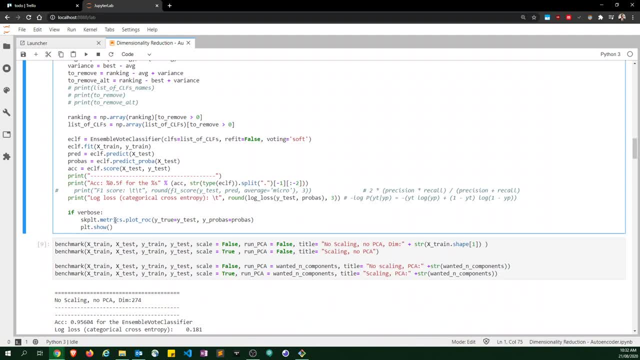 Verbose will basically control whether we print out a plot ROC. This is from a custom package, Because this plot ROC allows us to to plot it in our plot it when we have multiple lines to make. I will display this in a moment. 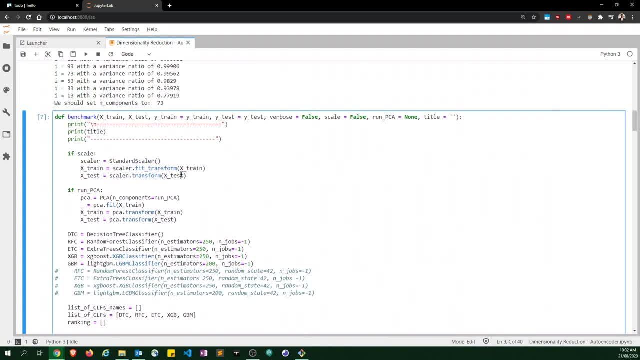 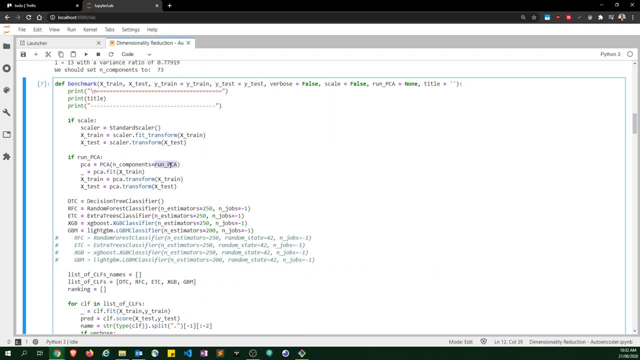 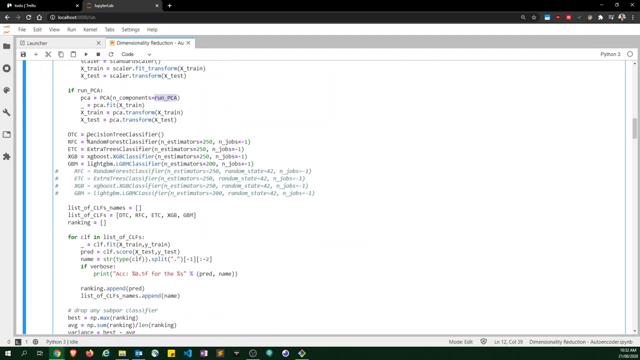 So basically, if scale, we scale our data. If PCA, well, if PCA is not done, we put one PCA over here And we scale our data accordingly. We have five classifiers And I have the n estimators pretty high. 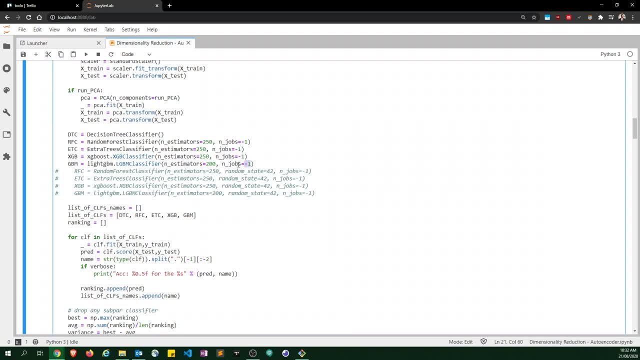 And I have the n drops set to negative one, which is to utilize all my calls. I have adjacently powerful computers. I can do this. If your computer is weak, you should probably leave it at default. Perhaps even for these two have it a little less than default n estimators. 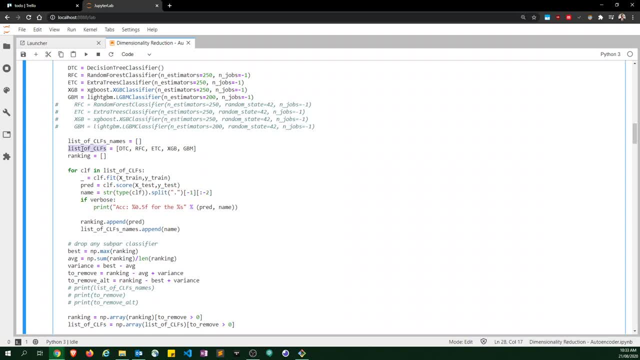 I went through a loop of the set of all estimators. Well, this is technically a list And I fit it scored printed out. I append the rankings to a list of rankings, which is just an ordered list, And I keep a list of the names of it. 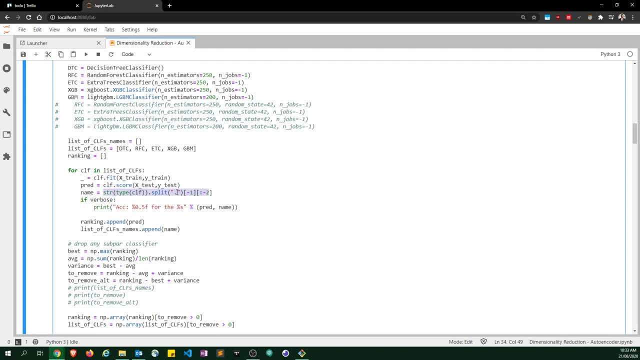 Because I'm doing a tiny bit of computation to find out the formal type of the classifier, Which would be like which at the, which would be a bunch of stuff, And at the end it would tell us: let's actually choose classifier. 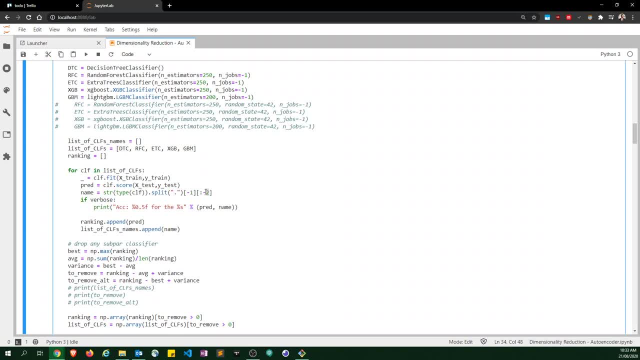 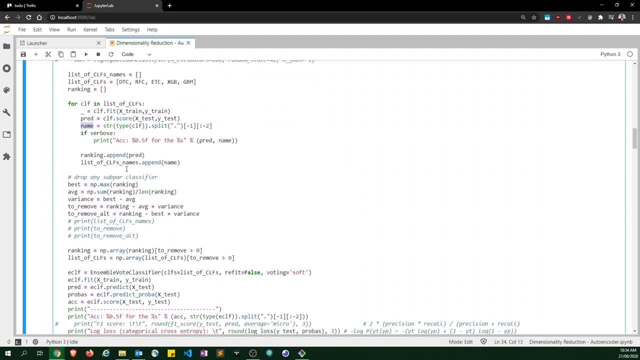 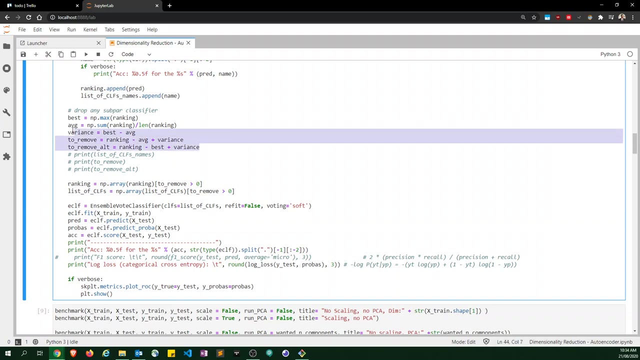 I just split it by zeros, get the last element, Strip off some unneeded underscores And that's how I programmatically get the name of the list reader. So in the classifier I'll do a little bit of math that I won't bother explaining. 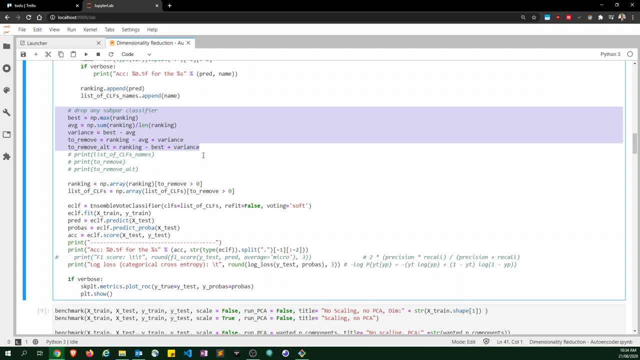 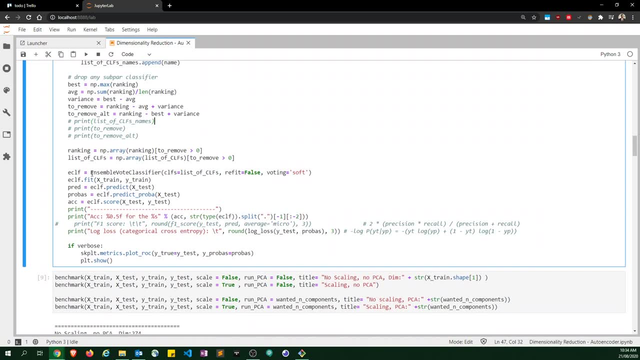 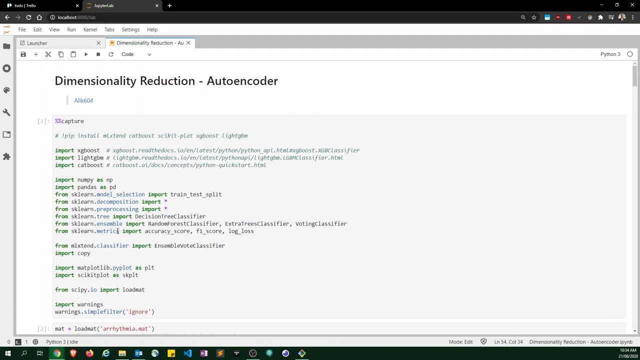 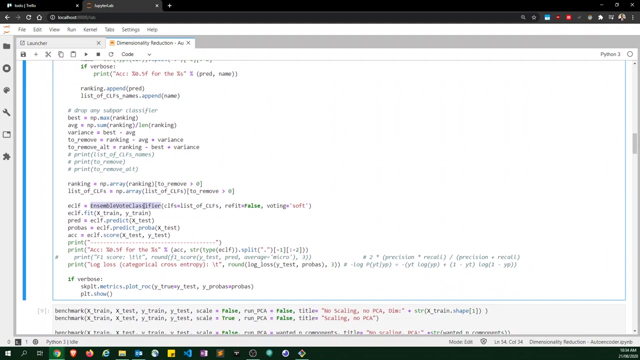 To drop any subpar classifiers. In practice, it removes the weakest classifier And I run this pack code Ensemble vote classifier, which is from the following package: ml-exchangeclassifier. Basically, this allows me to have an ensemble voting classifier. 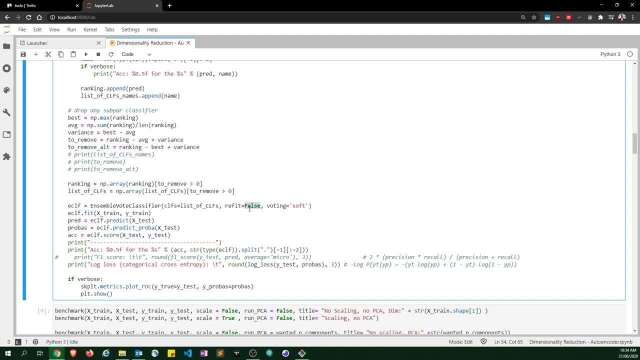 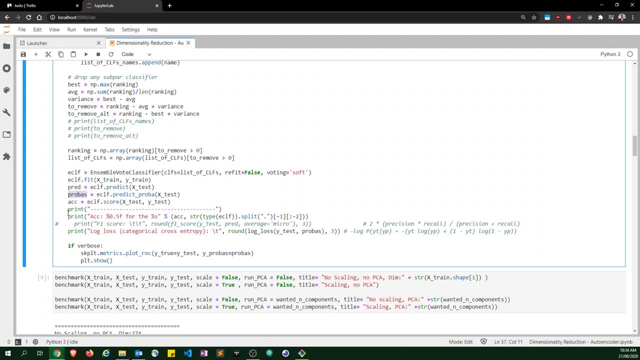 In which I can have refit equals to false. I don't want to do extra work. I don't have to Now. I get the predictions, probabilities And I just print out some basic metrics. In particular I get, I print out the accuracy. 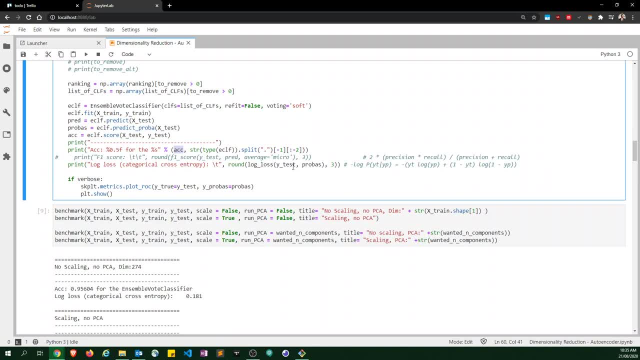 And I print out the categorical cost entropy slash, the log loss, Which is defined by right. here I could print out the F1 score, But in practice it ends up being exactly what my accuracy is every single time, Even though F1 score is defined as the following: 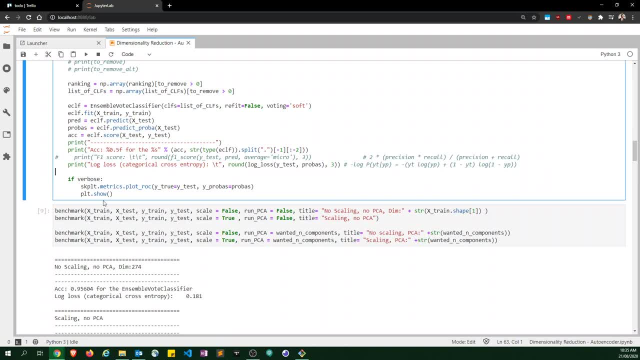 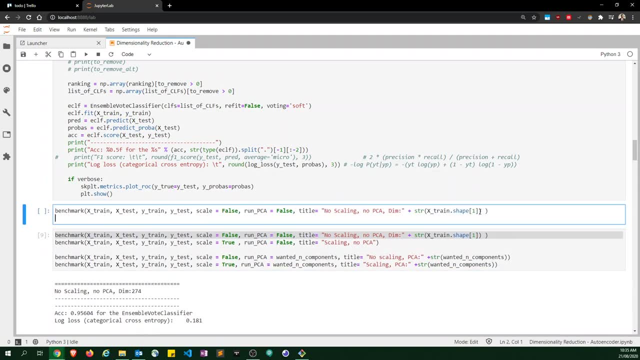 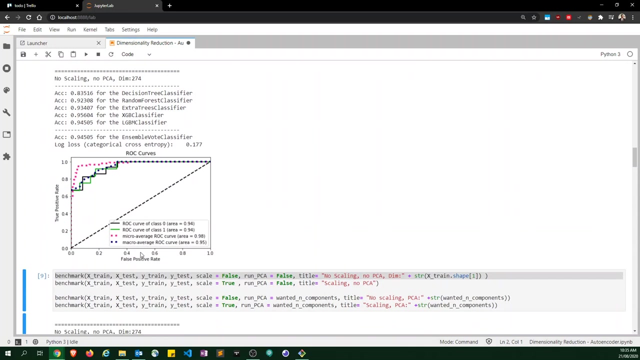 And Burbose prints out the plot ROC. Just for the sake of example, I will show Burbose. So this is what the ROC curve looks like. It's listed for class 1.. For class 0. And it goes through the micro-average and the macro-average. 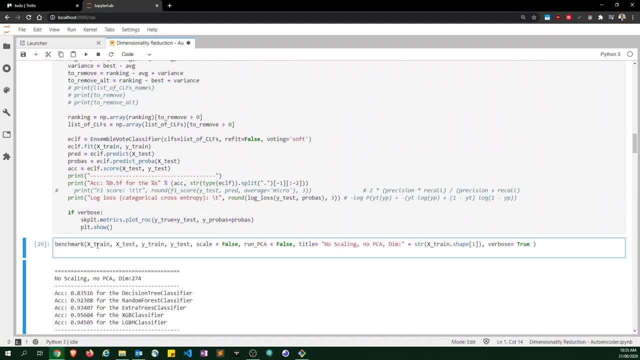 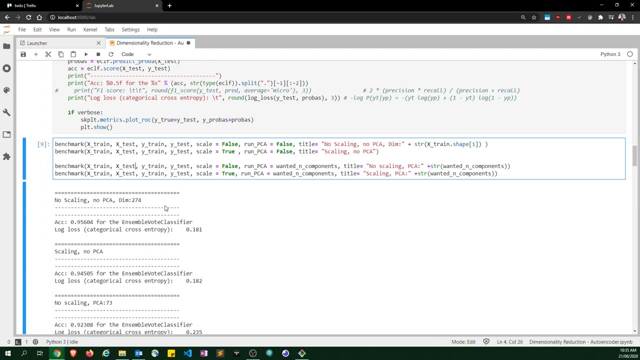 And, And, And, And, And, And, And. So you can just left click on any one of these. So I continue to show two. match up data noodle. alors non pratiquer Allright. So I call this benchmark several times. 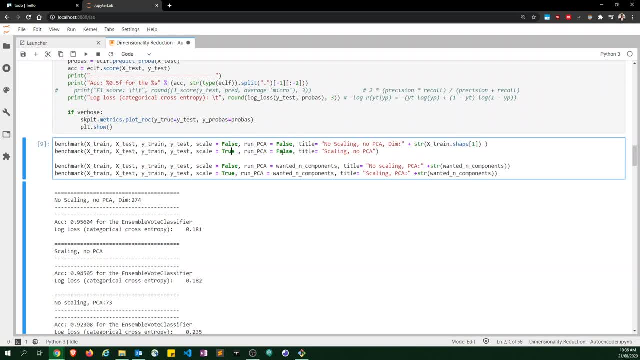 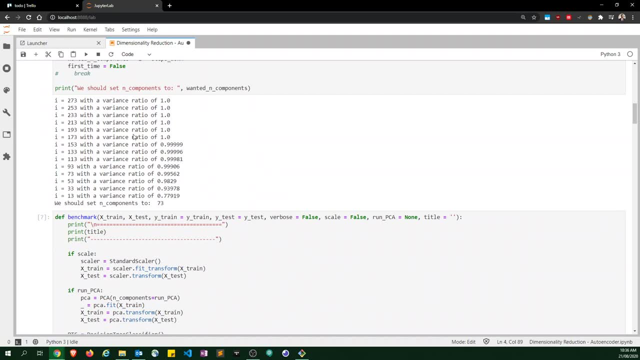 I do it edy, without scaling, Without PCA, With scaling Without PCA, Without scaling, Without scaling With end components, Which explains Which is the lowest number of end components when we are stepping down by 20. That still gives us a 99% experience. 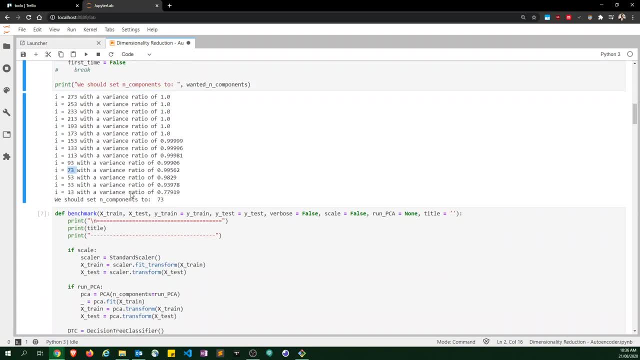 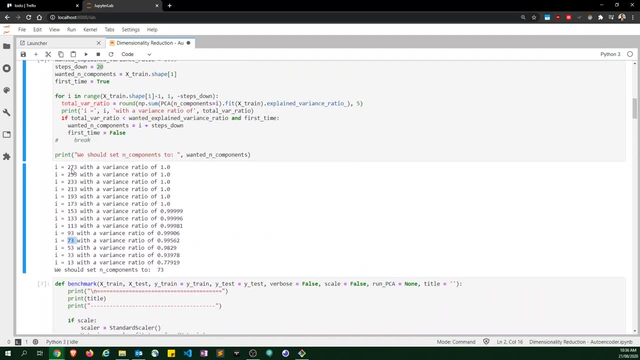 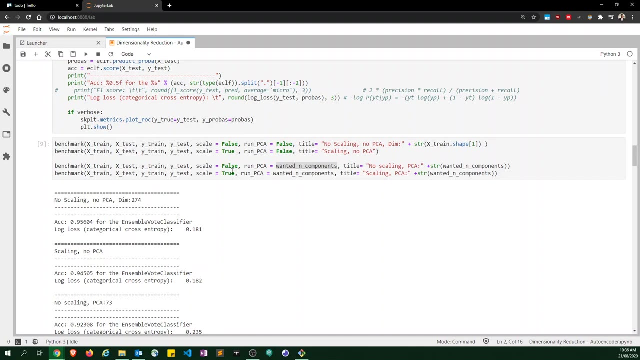 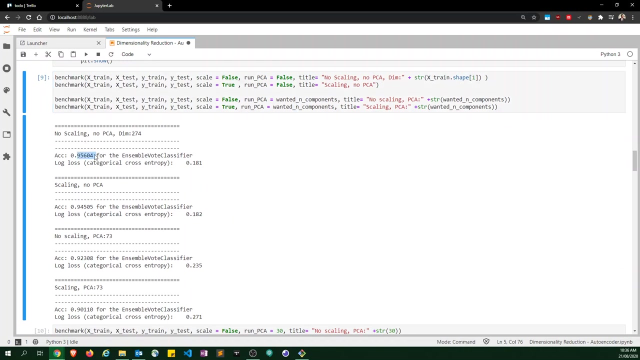 This can't explain to very much. visual, which is 73 in this case. In other words, we reduce our dimensionality from 273 down to just 73 and I sort with scaling and with PCA. So our baseline, without any scaling, is 95 or 96% accuracy. and if 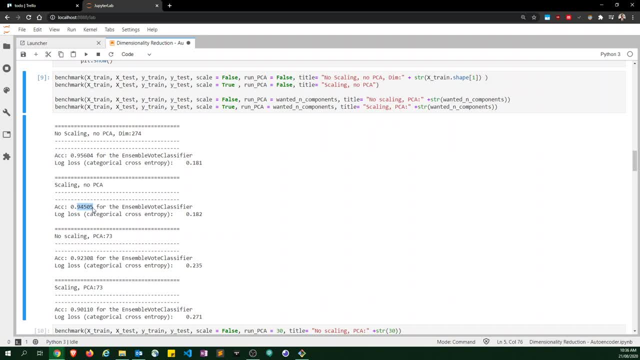 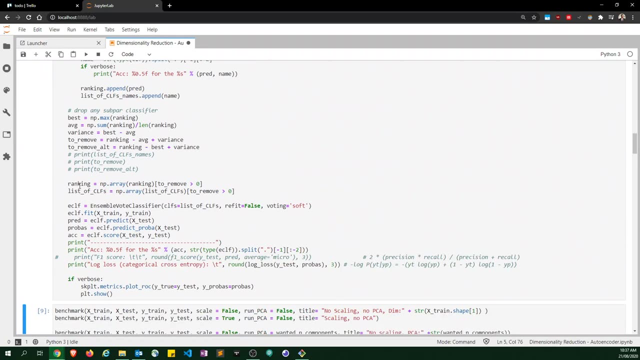 you do have scaling will lose 1% accuracy. Now, if we have no scaling and we have PCA, we will have 92% accuracy. Meanwhile, if you have scaling and PCA, you have 90% accuracy. So for the type of tube based methods, 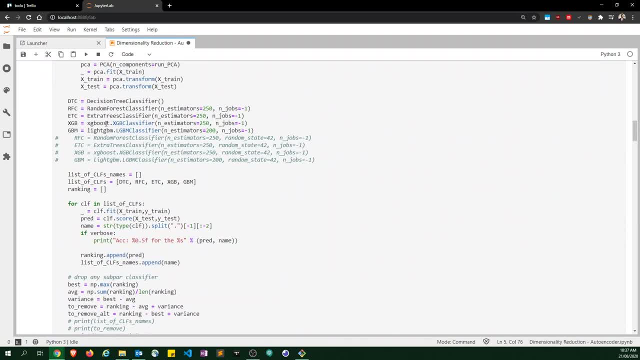 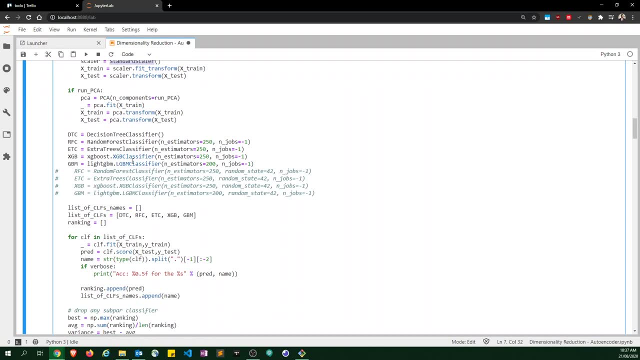 that we are using right here. we actually find that scaling will actually reduce performance, In particular, standard scaling- min-max scaling most likely would have 90% accuracy- marginal impact and the thing is this might be just due to the random state. I removed a random state for testing the auto encoder down below in which I used 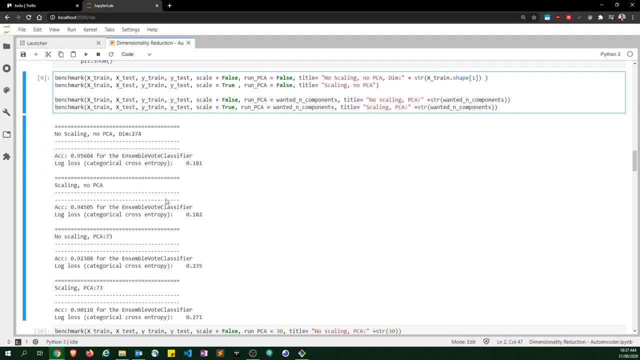 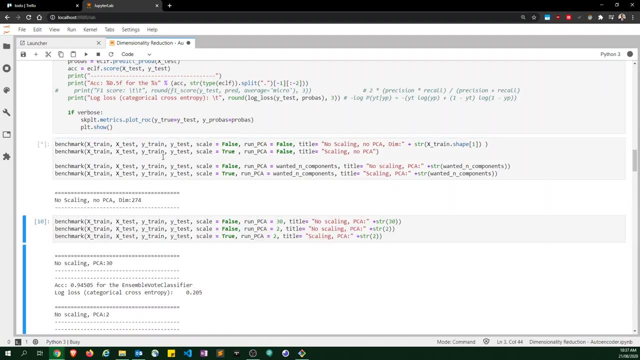 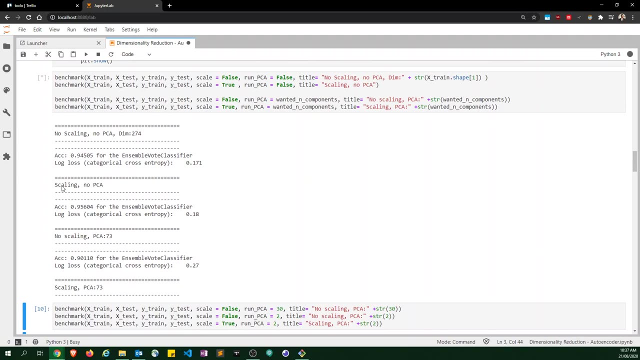 this code. but when I did use a random state, the spread between these was much less so scaling when I have a random state didn't matter very much. I'm just going to run this again just for a sick example over here. we find that scaling did actually. 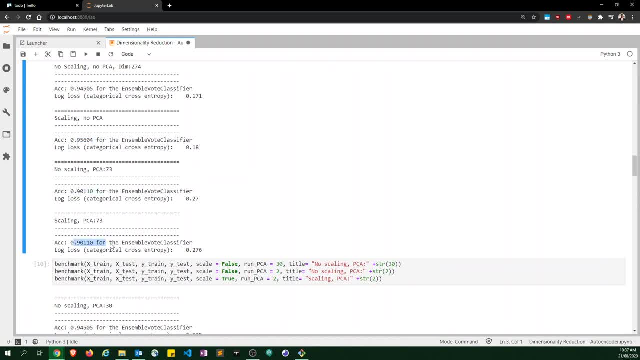 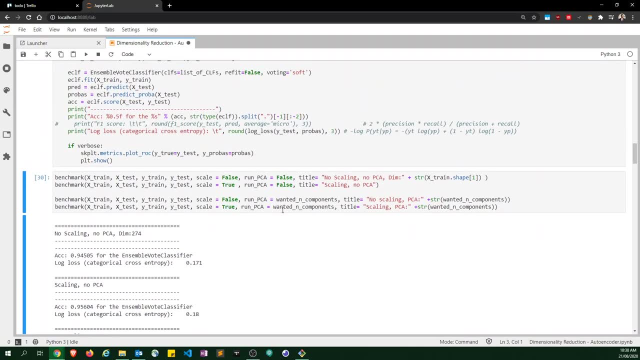 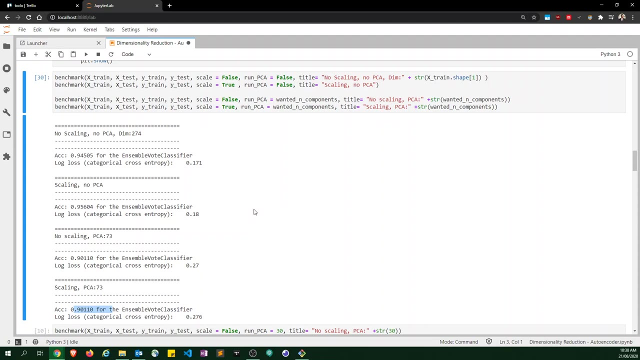 made a small improvement and scaling here actually didn't actually have an impact. so when we're scaling to 99% explained to entity, so it has a marginal impact. sometimes it's better, sometimes it's worse, but on average it's more or less the same. now I went some the same. 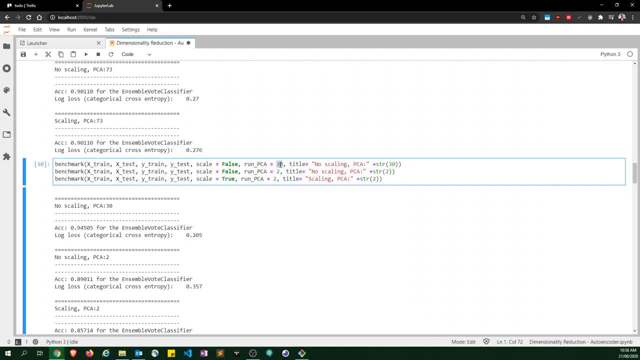 besser, we go back to the scale from the previous example. so we go back to our benchmark without scaling, with PCA equals 2, PCA equals 2,- sorry- PCA 1, PCAs and components equals 30 and components equals 20, and with scaling, PCA and components equals 2.. 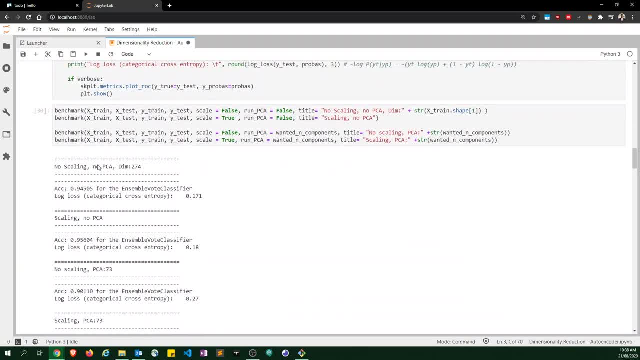 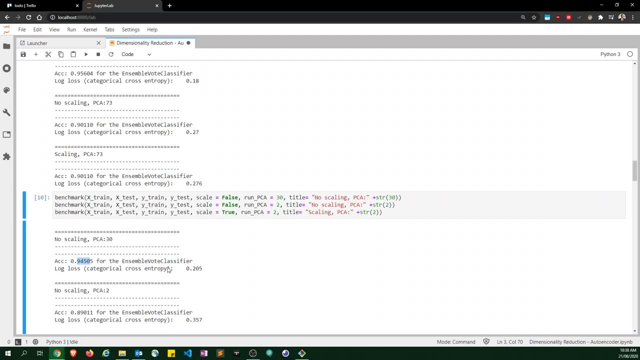 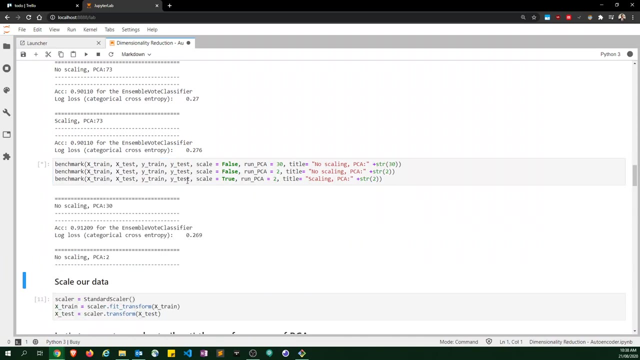 So we got 94% accuracy, meanwhile up here we were getting about 90% accuracy, which is weird. we have less components but we have higher accuracy, which is, like, really weird. but that's what I got and I'm quite confident there's not a bug in my code or anything like. 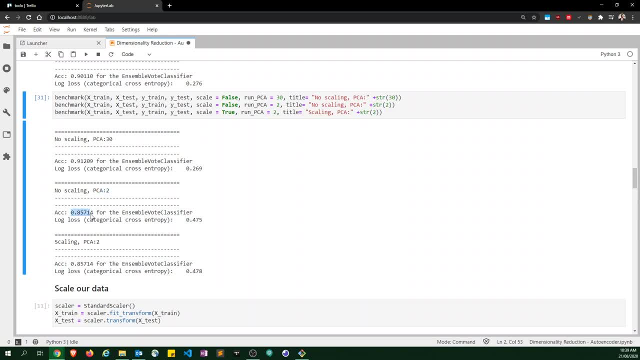 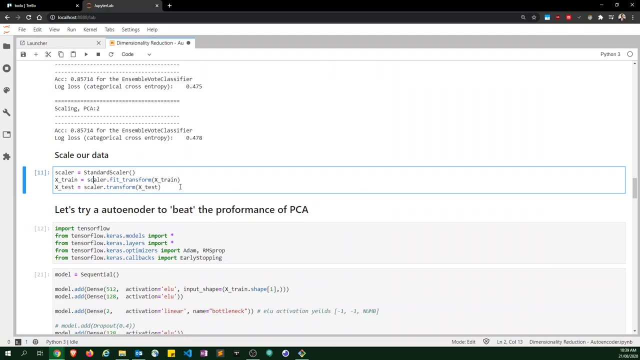 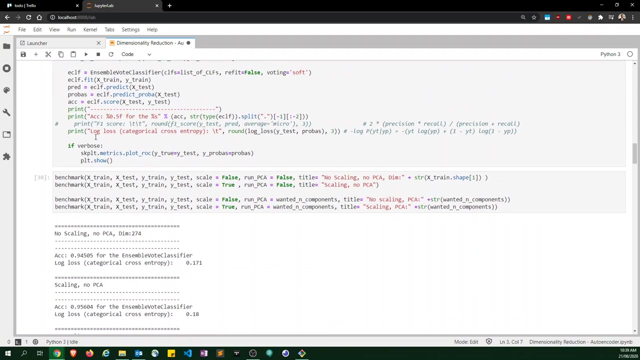 that, And when we have PCA equals 2, we get 85% accuracy. and even if we have scaling, we have 80% accuracy. In my past testing I found out that this is not always the case. We scale our original data one more time because now we no longer have encapsulated enough. 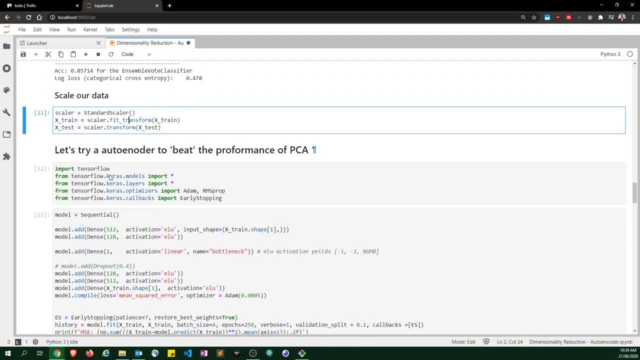 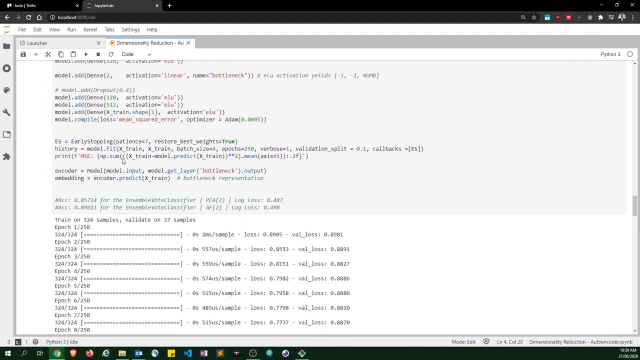 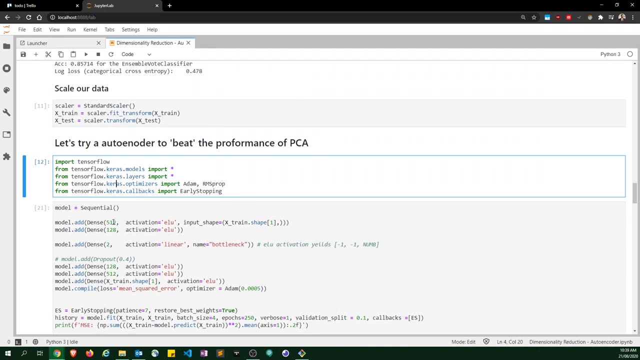 function. So for the neural network, I want everything to be scaled. I do some basic imports with tensorflow 2.0.keras. I define my autoencoder. It will start off with 512 units, step down to 128,, step down to 2.. 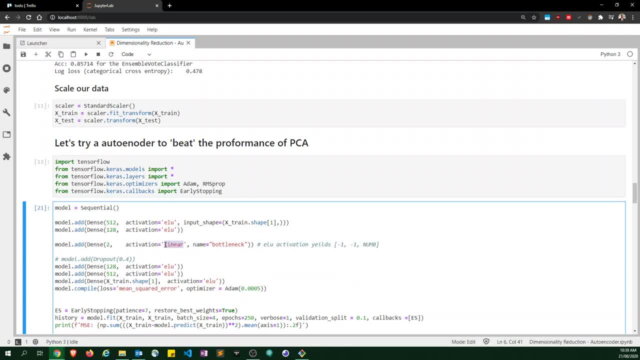 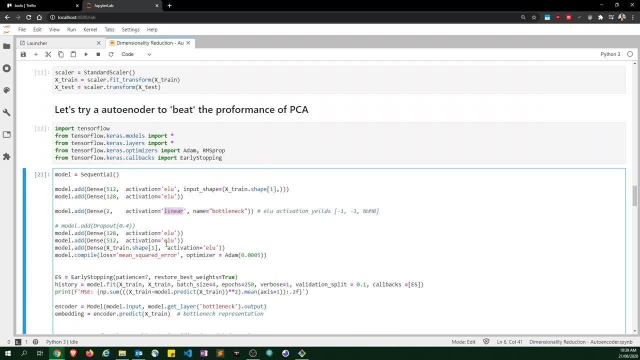 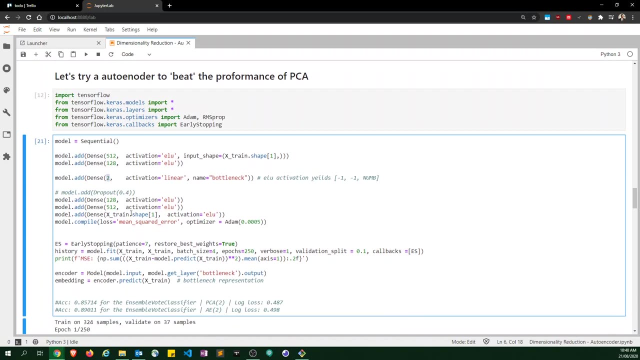 This. I keep it at linear. It just helps it a whole lot more. if I have it at something else, The autoencoder will try to. basically one of the features over here will end up being 0 typically, and I find that to be a huge problem for the purposes of dimensionality reduction. 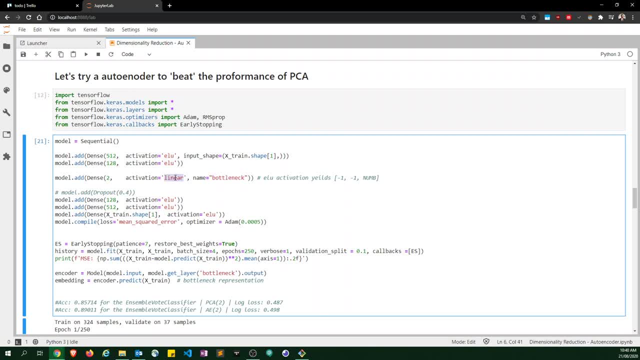 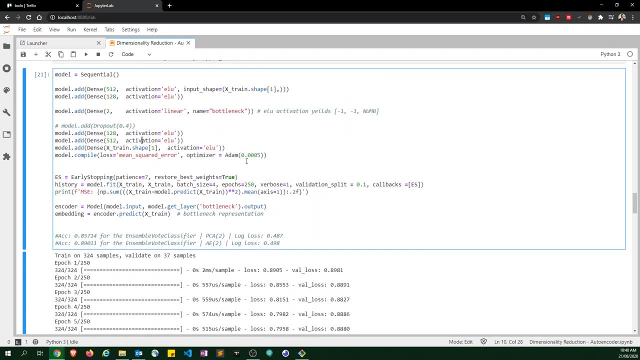 It's best to keep this at 0, even though you might be able to get away with 0 or something else. I will use that opposite sequence to step it back up. I use Adam with half the default loading rate. I have only stopping with a patience of 7.. 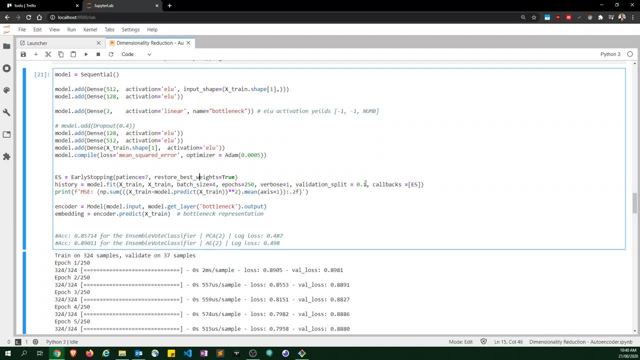 The store best rate is pretty normal. I have a validation split of 10% just for the sake of metrics. I have a very small bat size and a very high number of epochs, but that doesn't matter because I'll stop when I converge. 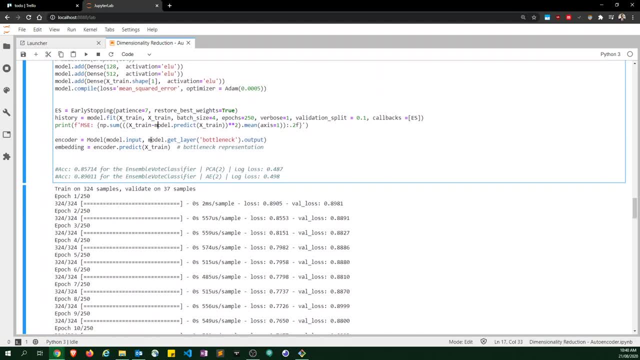 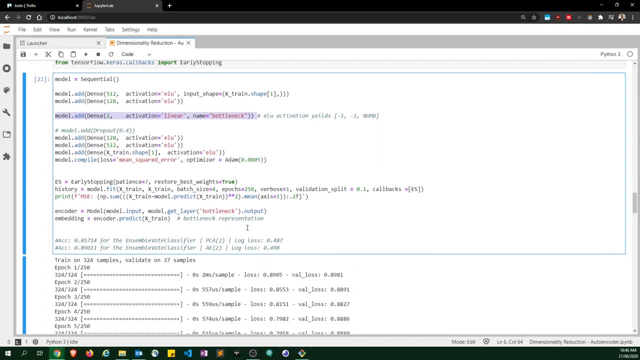 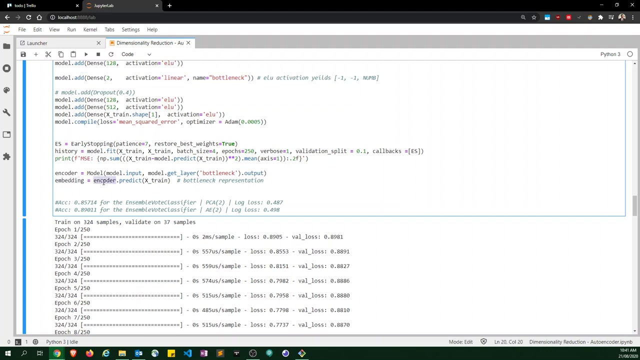 I'll stop when I converge. I have my encoder defined to model input comma get layer bottleneckoutput. bottleneck is, of course, this point in which we have two feature vectors in our neural network. We have our embeddings, which is just encoderpredict xchain. 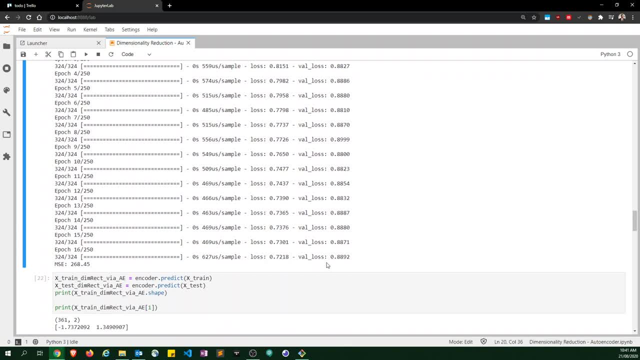 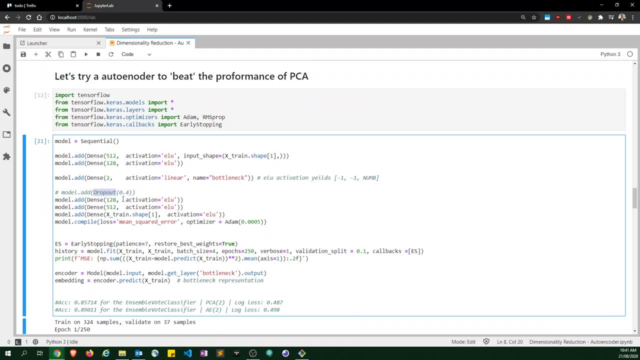 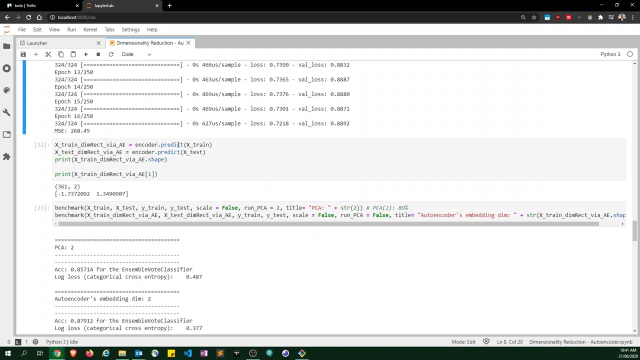 So I run this code And I found out: okay, we're overfitting a little bit, but I'm not going to worry much about that. I did test it with dropout, but I decided to not bother with dropout. So I predict with the auto encoder, the xchain, the xtest, and I print out the dimensions. 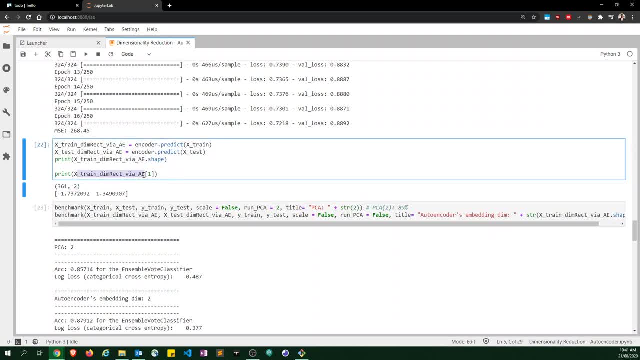 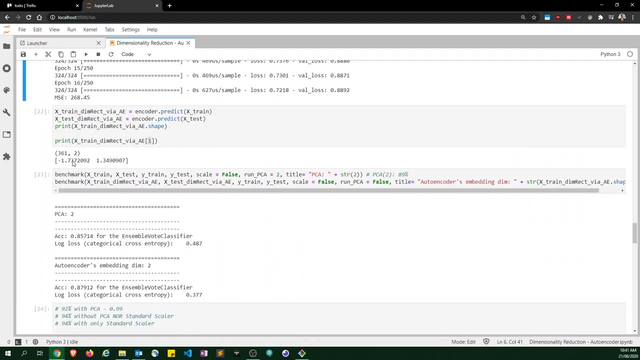 We indeed have two feature vectors, And I print out the first chaining- It's the xtest, And I print out the dimensions. And I print out the second chaining, sample of data. And the main thing is these two are integers. If this was to be elu or something, sorry, these are real numbers. 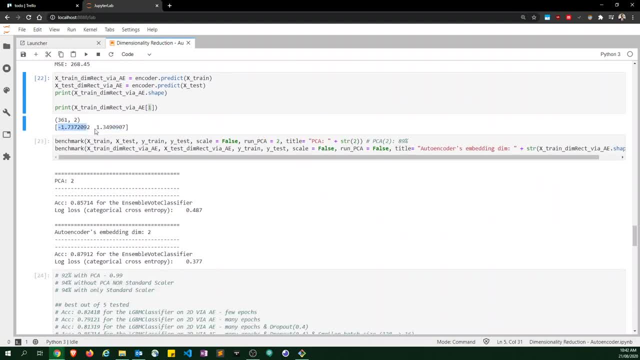 If that was, there was to be elu, then one of these could be zero, And in my testing I found that actually just happened. So that's why it's best to keep it as linear. We run our benchmark without scaling, because I found that scaling for PC2 was harmful even. 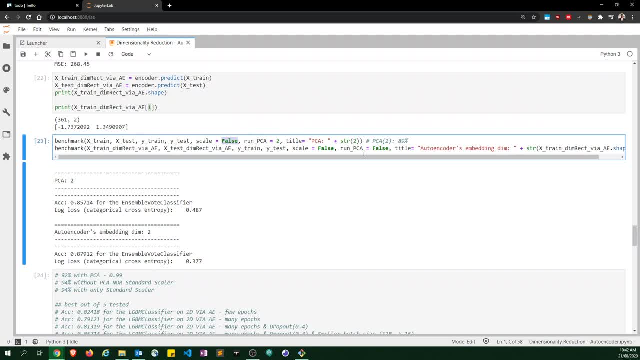 to our benchmark, Even though I couldn't show it up above, And our PCAs and components will be equal to 2. And I run benchmark with our xchain and our xtest from our auto encoder. We do not scale here either. 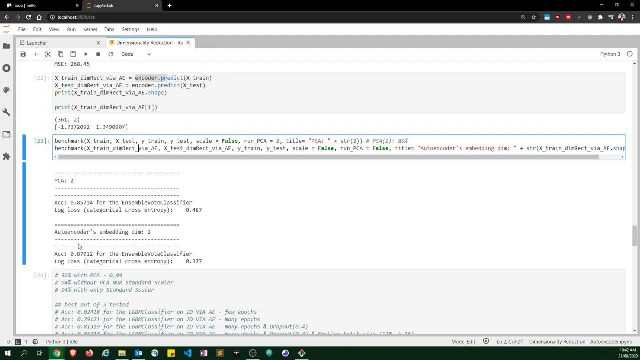 And we just print out a title to make it extra clear. And I run this And I found that our auto encoder gave us an error. And I run this And I found that our auto encoder gave us an error And I found that our auto encoder gave us an error. 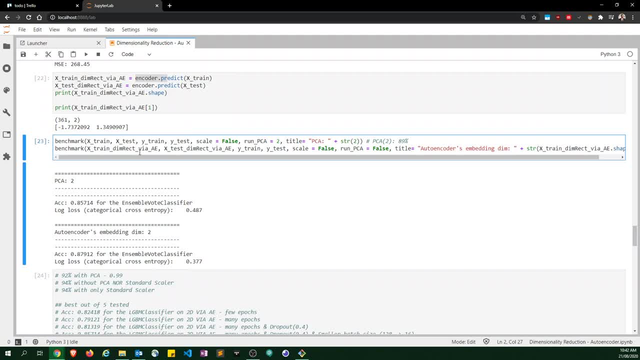 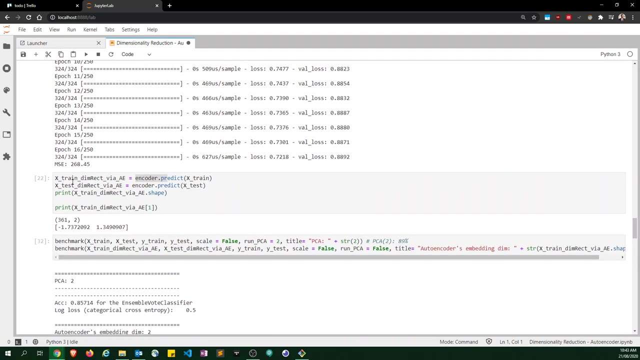 And I found that our auto encoder gave us an error And I chose to save better accuracy and a lower islog loss. This doesn't happen all the time, but this occurred due to the change that I got. So, yes, I did arguably run an informal gridsearch on the bender이�ntebed, which is: 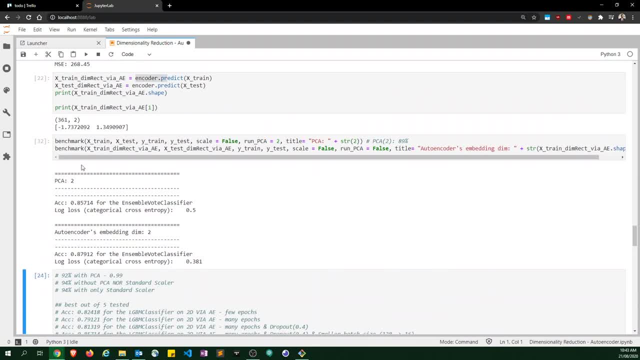 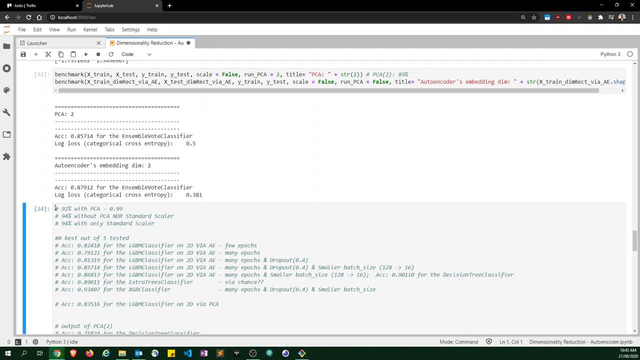 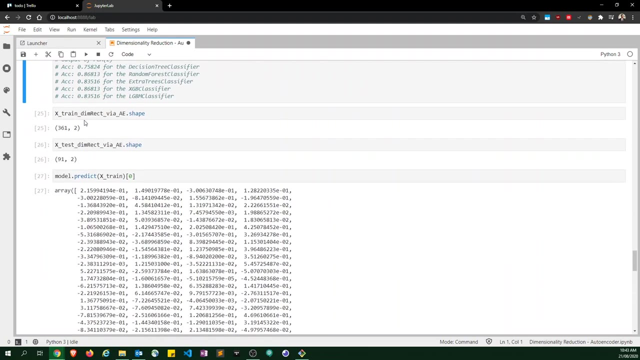 really a meme in academia, But this does so that it'll indeed work, Even though it may not be easily re-creatable- have to run the directory code a few times or figure out any more superior model architecture for this. Below I just have some random debugging stuff that doesn't. 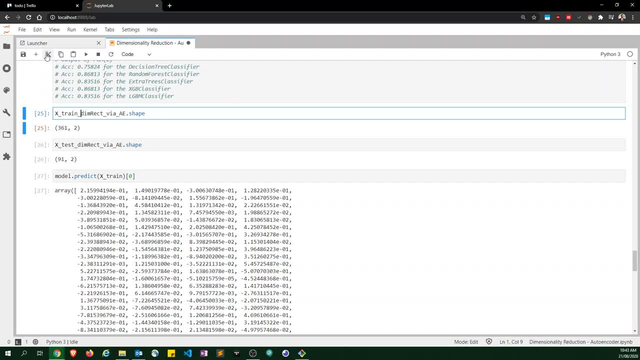 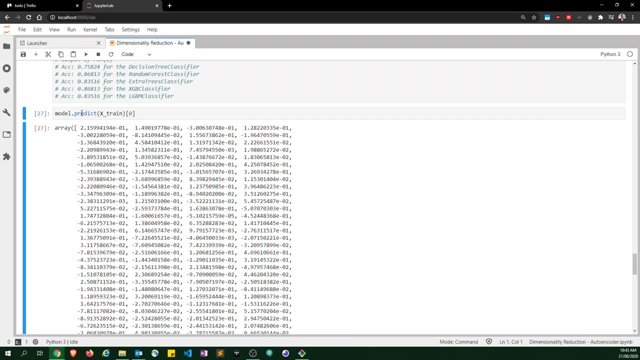 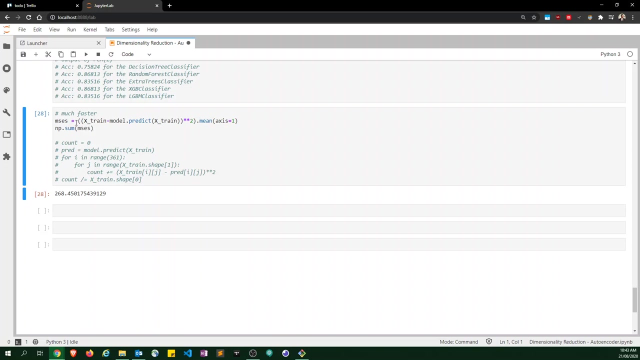 actually matter. I just wanted to show that the number of samples here is 361. for a test it is 92, 91, and if I was to predict my x-train, I would get numbers that look like the following and, just as a closing note, I actually found that: 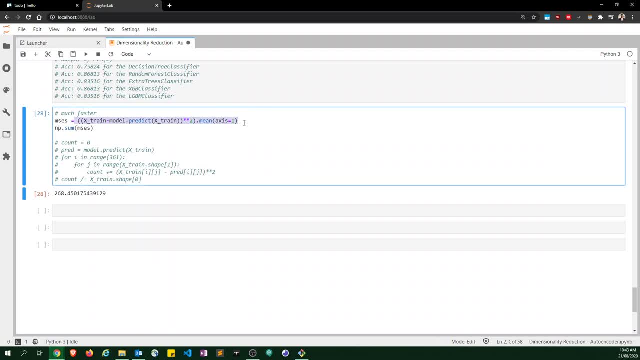 computing the mean squared error myself. its actually very fast if I do it in this way. it's faster. if I was to use S-Clay lines and if I were to compute it in my own, these classical double-folded loop type ray, It would actually be relatively 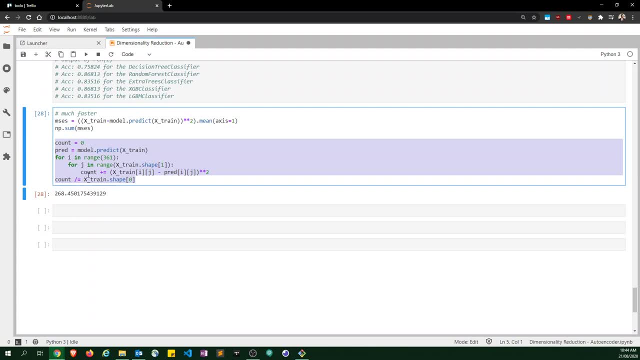 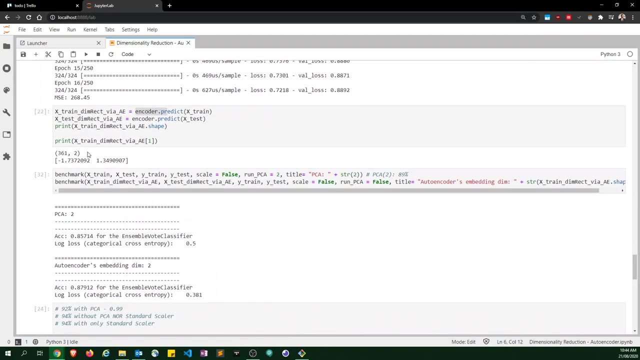 fast. so double full loop is much slower than actual zero. So double full loop is much slower than actual final level in which is slower than using it doing it by this way. and that's it for the video. if you're interested in the way I present content and the fact that I